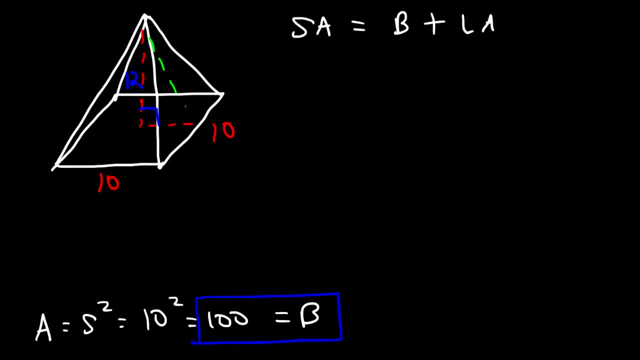 notice that this forms a right triangle and this represents the slant height. now, if this is 10, that means this section here has to be 5, and so if we focus on that right triangle, if this side is 5 and this is 12, we have the 5, 12, 13 right. 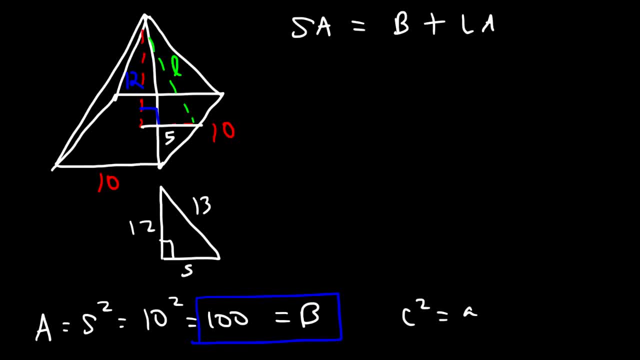 triangle and you can use the Pythagorean theorem to get that answer. so C squared is equal to a squared plus B squared. a is 5, B is 12, 5 squared is 25, 12 squared is 144, and so C squared is equal to 169 if you take the square root of 169. that. 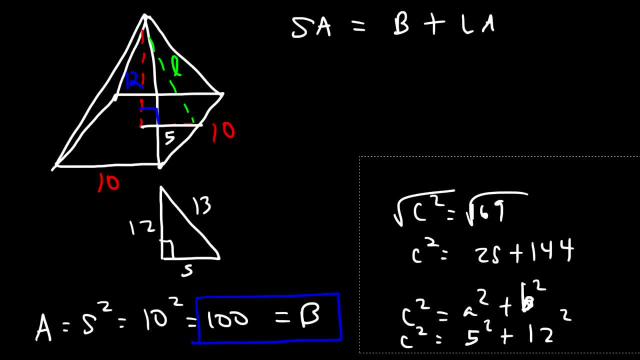 will give you 13, which is the slant height. so this triangle here is basically this triangle that you see right here. it's one of the four triangles. so we have the slant height, which is L. that's the height of this triangle. that's 13, and the base of this triangle is 10. so now we can. 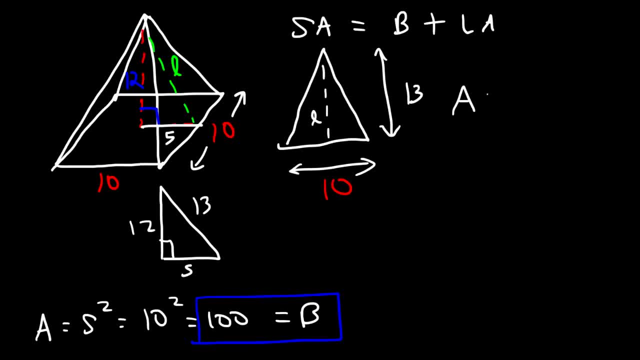 calculate the area of that triangle. so the area is going to be 1 half base times height. so the base is 10, the height is 13, half of 10 is 5, and 5 times 13 is 65. so that's the area for one triangle. the lateral area is going to be the total. 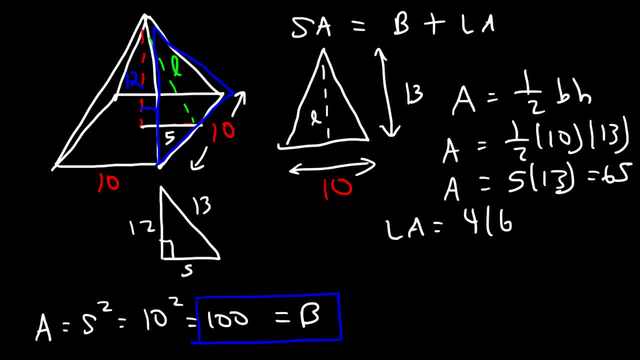 area for all four triangles. so it's going to be 4 times 65, which is 260. so that's the lateral area. so to calculate the total area, it's going to be the area, the base, which is a hundred, plus the lateral area, which is 260, so that's going to be 360. 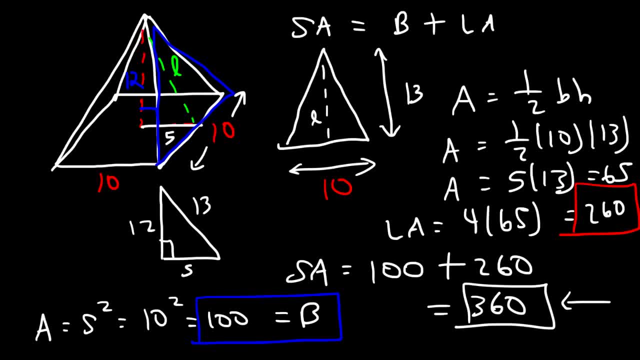 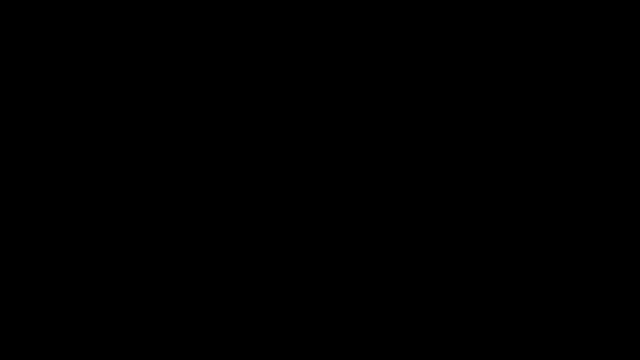 square units. so that's how you can calculate the total surface area of a pyramid. so that's how you can calculate the total surface area of a pyramid.